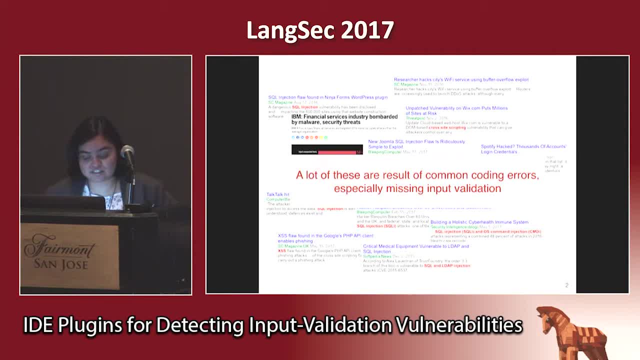 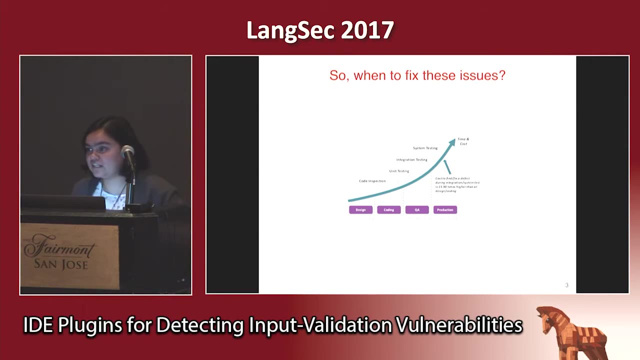 them are result of injection attacks resulted from missing or incorrect input validation. So what do we have to what we can do about to solve these problems? So previous research showed that it is become more costly and costly if we want to try to fix this at the later. 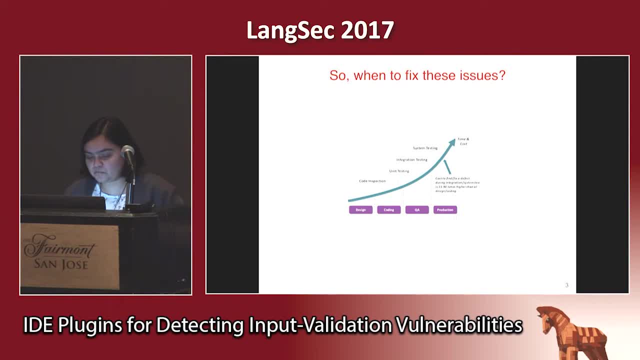 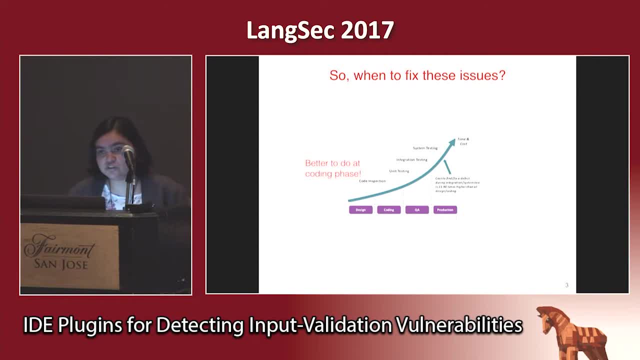 So in this talk I am focusing on how we can e-cube the code. So we have developed developers with tools more friendly to use and we are to encourage them to have secure coding practices. So we know there are a lot of static and dynamic analysis to available. So what's the problem? 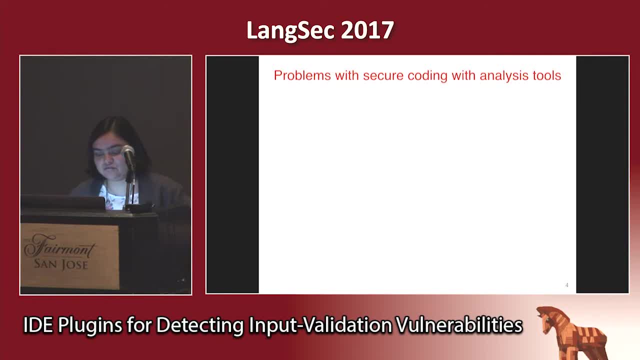 with those to use those at the coding phase. So previous studies showed that some developers have concern that if they need to, it's use a separate tool to do the analysis. it disrupts their workflow. They need to move back and forth between their IDE and the tools they are using to check security flaws Also. 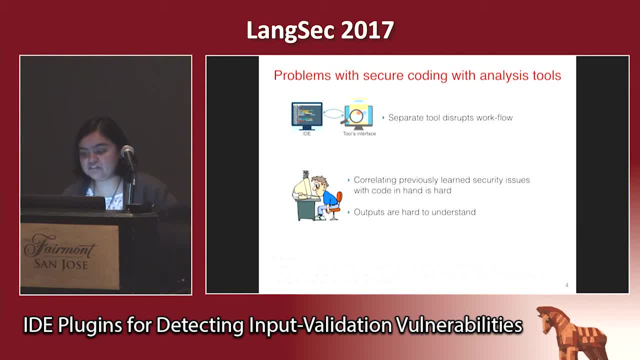 there were some complaints about correlating previously learned security issues with coding. hand is hard and also the outputs are hard to understand. So we are thinking it would be better if we can incorporate the security analysis with the IDE. then there is no context switch. 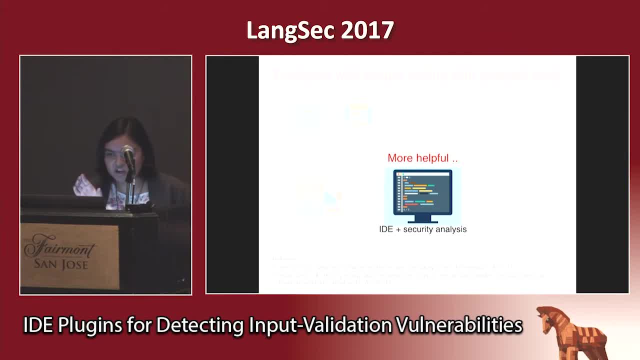 So we are thinking it would be better if we can incorporate the security analysis with the IDE. So if we get the security information, flaw, information just in the code which is causing the problem, then it would be better to understand and fixing those. So what did I mean by incorporating security analysis in IDE? So in recent days there 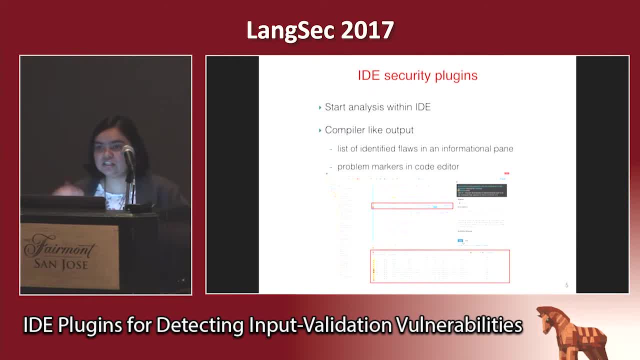 are some plug-ins available that you can include in your IDE. Then you can start the static analysis within the IDE like a regular button press, like how we start the compiler. So there is a list of flaws at the information pane at the bottom and also the line with 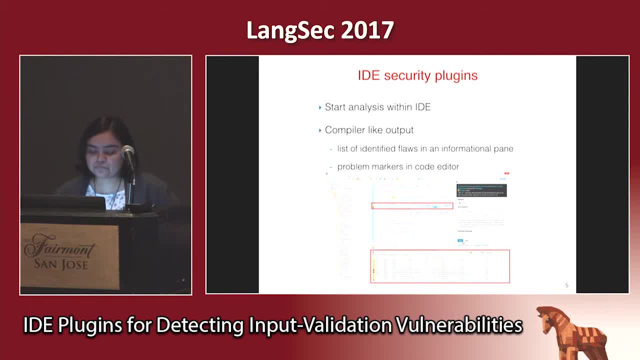 the problem has some problem markers with it, So this type of feedback is quite common to us. We are more familiar to us, so it will be more helpful to have this kind of feedback. So we are thinking it would be better if we can incorporate the security analysis with the IDE. then there are some plug-ins available that you can include in your IDE. Then you can start the static analysis within the IDE, like how we start the compiling, and then it shows the analysis result like the common compiler errors. So there is a list of flaws. 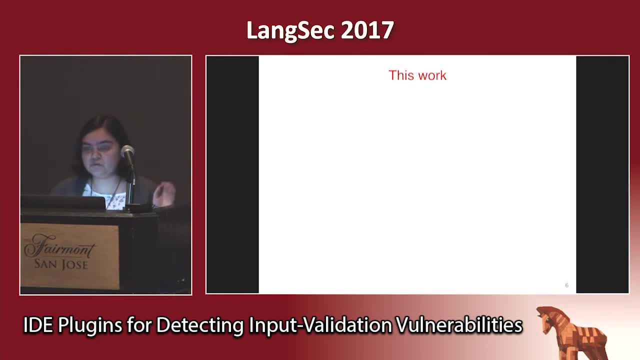 that we have used for not having those kinds of functionality. So in this work we did a review of such available IDE plug-ins that have security functionality. So we tried to find out if they are available, whether they're free or commercial, if we 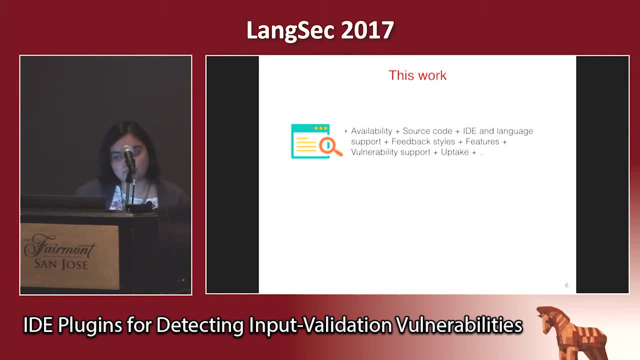 have a tool or not, what IDE language they support, what type of feedback they provide and if they have any additional features or which functionality they can use. and then vulnerability checks they performed and are they popular or not, stuff like that. 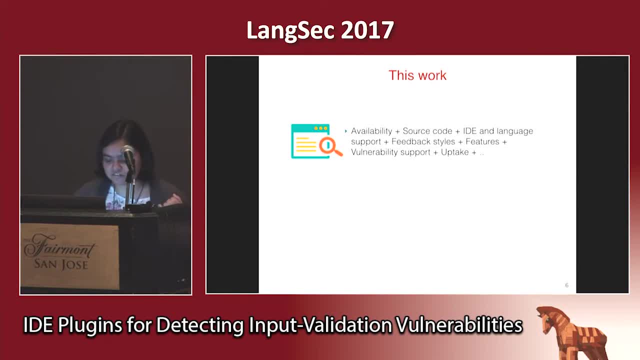 So how we did it, so how we built the list of the plugins that we want to study, is like we went through the listings of plugins from different IDEs. We also look at the static analysis tools to check if they have any plugin version of. 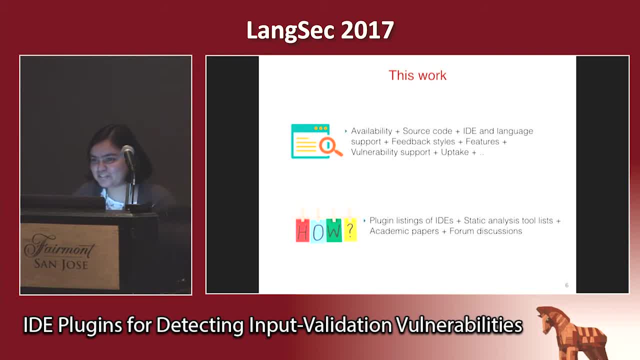 it available. We also check- obviously check- the academic papers and also we go through the forum discussions to check if people are talking about some plugins. So for this work we focus on input validation related vulnerabilities and also we wanted to do this from a perspective of a regular developer. 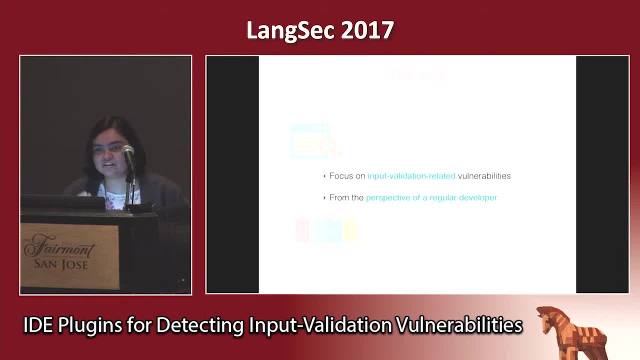 So to understand what the problem they face to gather information about these plugins, Okay, So so this is what we got. We got total 17 plugins. Four of them were from academic studies. Let's look at some more information about them. 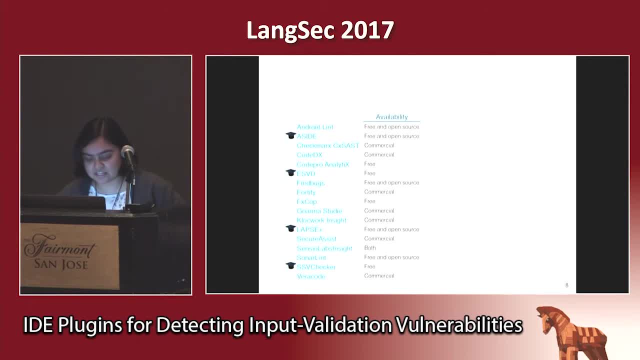 So here are the availability information of all these plugins. So how easy or hard to access security plugins? Not hard, we can say There are some. there are nine free plugins available and five of them are open source. So if developers want to dive more into how these plugins work, they can do it. 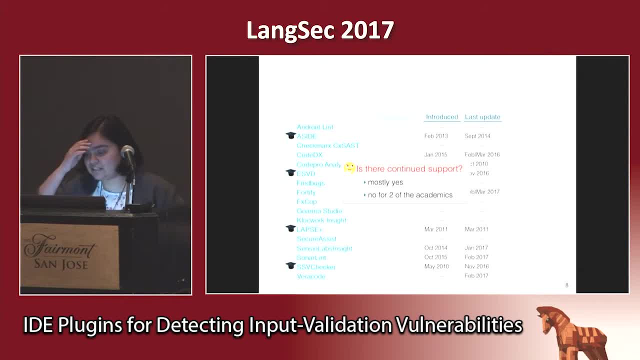 Next we looked at their dates introduced and last update to check: is there continued support for them? We can say mostly yes, Not much for the academic ones. But another thing to note that's like it doesn't necessarily mean that no, recent update does not necessarily mean 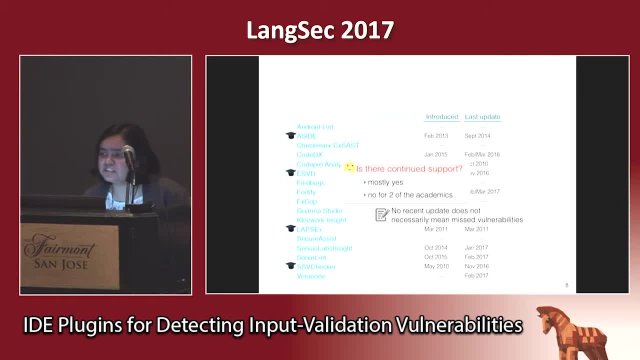 That there are missing vulnerabilities, because some of the problems are still valid. They are not totally obsolete. So this skill injection or cross site scripting the definitions is not changing that much. Okay, So here are the information about the supported IDs and languages and platforms. 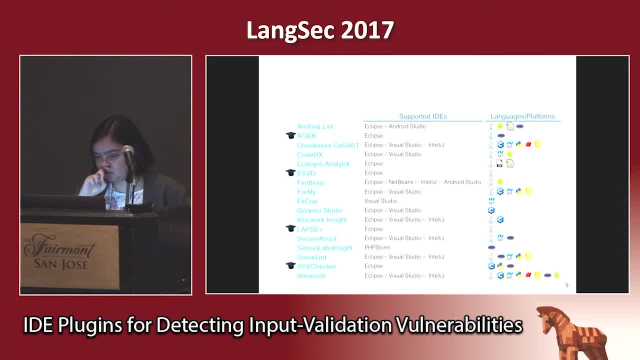 So a lot of them are Eclipse plugins and we also have a lot of Visual Studio and IntelliJ- Mostly Java support, but we also have C++, NET, Python, JavaScript, PHP. So the question we had: do these plugins support mainstream IDs and languages platform? 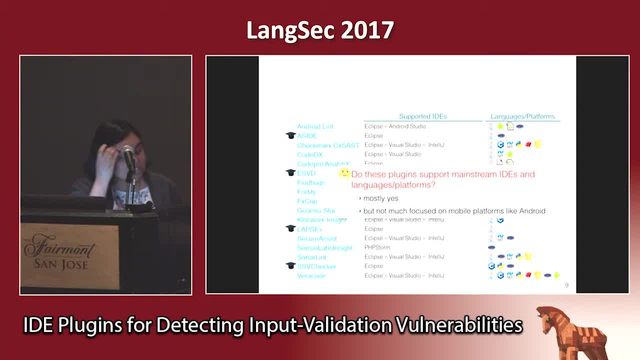 We can say mostly yes, But we are quite, but we are hoping to see more tools focused on mobile platforms, But we found only three that just focused on Android. Excuse me So what type of feedback they provide? So they provide the detective vulnerability description kind of varies plugin to plugin. 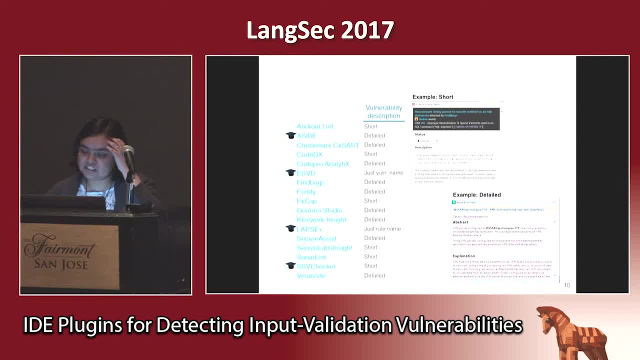 Here is two examples. The first one is quite short. It is just saying that there is a non-constant string in the skill statement and there is a chance of a skill injection attack. And the second one is quite long. It's saying that if there are 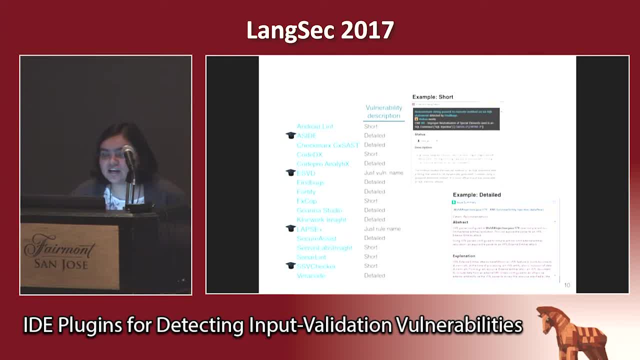 What did it mean by injection attack? So that means an attacker can have some malicious input and how it's going to affect it- A lot of more details, Not just saying that it is skill injection. So the next, if they provide any mitigation, not really. 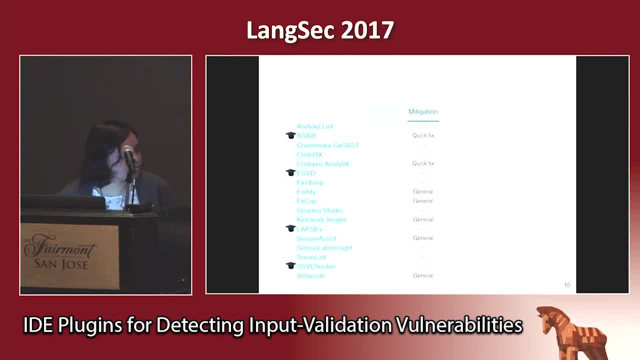 Couple of them suggest some code changes, but they are kind of general suggestion. Like: here is an example of parameterized query, something like that, And only few support quick fixes. that is specific to the code in hand. Next we check if there are any additional features. 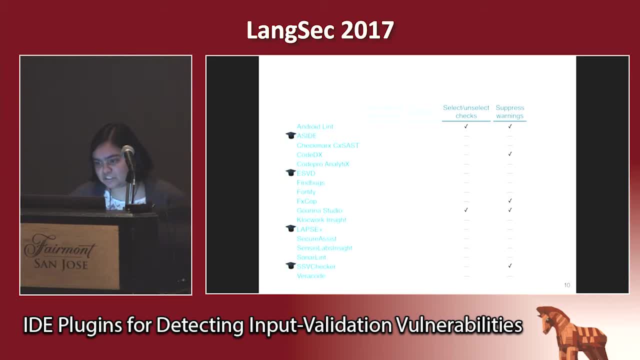 So we found that there are two features that this plugin supports: Select or unselect checks and suppress warning- But very few support these features. So these features are useful when the tools are generating a lot of false positives and in that case having a functionality like suppress warning will help the users to get. 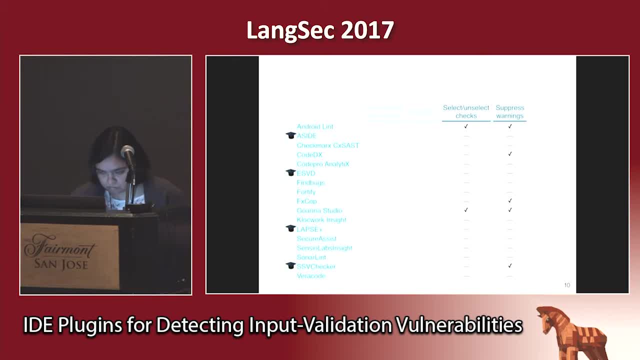 rid of that. So next, what vulnerability check these tools perform? So the top ones are all the input-related vulnerability that has support in these IDE plugins: Improper input validation, command injection, OS command injection, cross-site scripting, SQL injection, LDAP injection, smell injection and path injection. 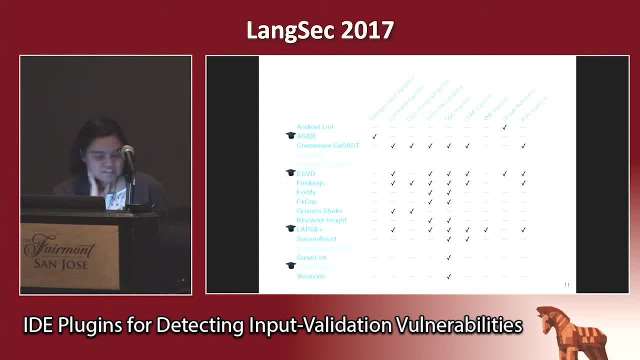 So, as you can see, not all provide support for all. You can see that there are some blank spaces. So for these two, they actually use multiple analysis tool and then provide a combined result, But a combined vulnerability check is not available, So we could not verify which checks they perform. 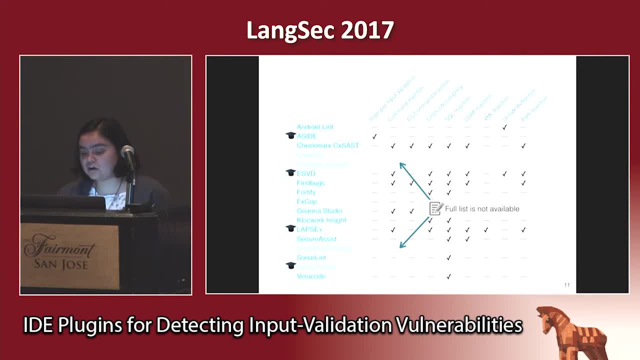 And for these two what checks they perform. the full list is not publicly available. So among these all checks, you can see that SQL injection is kind of the most common among all of them, And the next is cross-site scripting. Not as much as SQLI, but still quite good support. 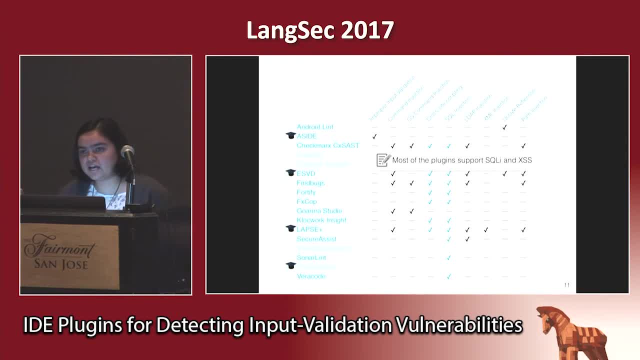 So I described what tools we found and what information we found, And I'm going to show you what tools we found. So the first problem: we noticed that, okay, there is no separate security category in IDE plugin listings. So if a developer wanted to use a tool, want to find the security tools they need to go. 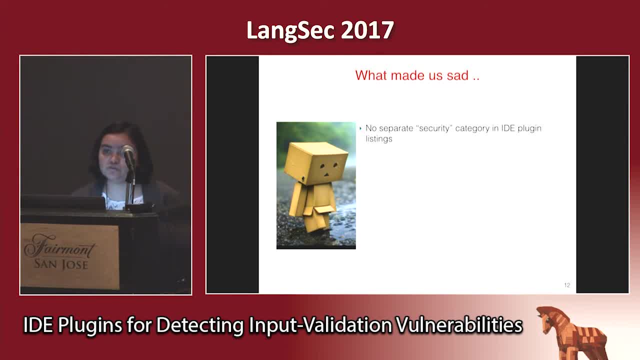 through a lot of code analysis tool to figure it out which one is actually provides security functionality. So the exception is Visual Studio. They have a security category, But most of the plugins at that category is primarily for code obfuscation and group code access. 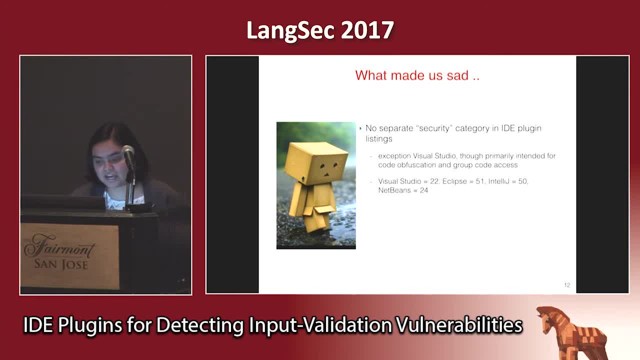 So it's not like that Visual Studio has a lot of categories compared to others. Visual Studio has only 22 categories compared to Eclipse has 51,, IntelliJ has 50, and NetBeans has 24.. But none of them were for specific to security tools. 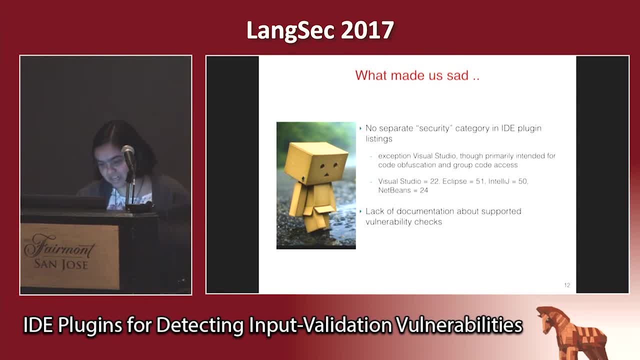 The next problem we think We found is like there is lack of documentation about the supported vulnerability checks. As you remember, there were some blank spaces about some of the tools And also the other checks. other information we gathered some of were very comprehensive. 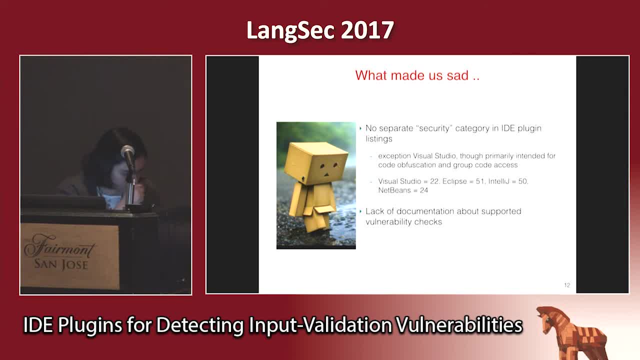 and they had CW. They have CW and CVEs, But others are not, So not that good to check what vulnerability they perform. The next problem is there is no way for developer to know how good or bad their detection performance is. None of them provide any benchmark results. 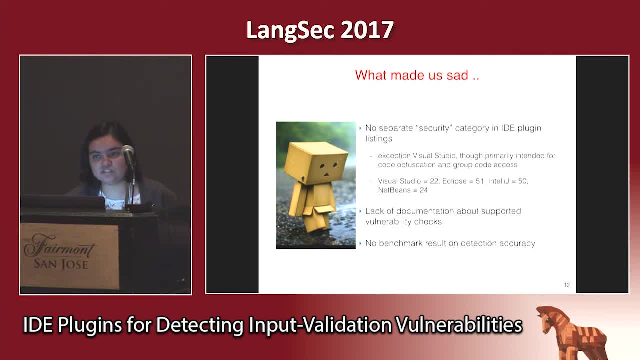 We found only one tool that provided benchmark result- again OWSP benchmark- But they, just a couple of weeks ago, discontinued the plugin support, So we Excluded that from our study. So this is what we did and what we found while doing this. 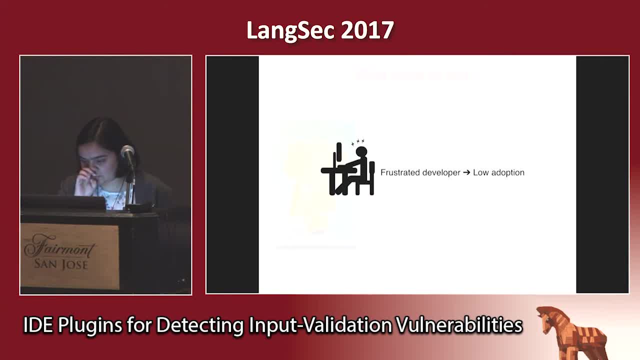 So this, And also we feel like how it made us sad, it will make the developer also frustrated and it will contribute to lower adoption. So what's next? So what we are doing, So what we are doing, So we are mainly interested in the usability testing of these tools.